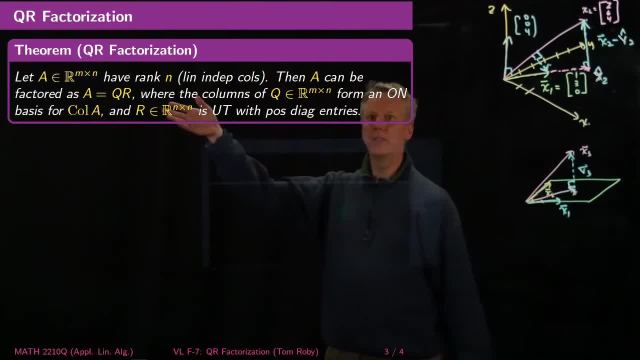 So suppose that here's the theorem. suppose I've got an m by n matrix. it has n linearly independent columns, so rank n. Then when I factor it I get this matrix: Q is in R, m by n and its columns are an orthonormal basis for the column space of A. So the way I'm going, 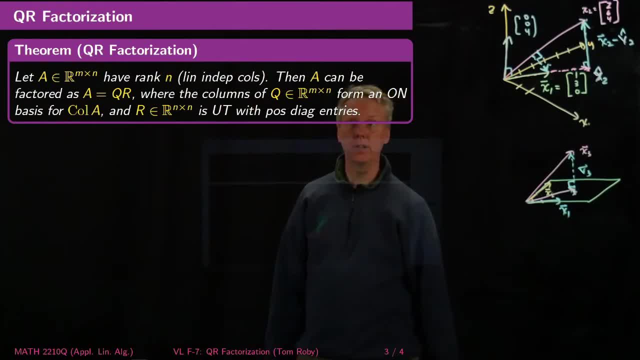 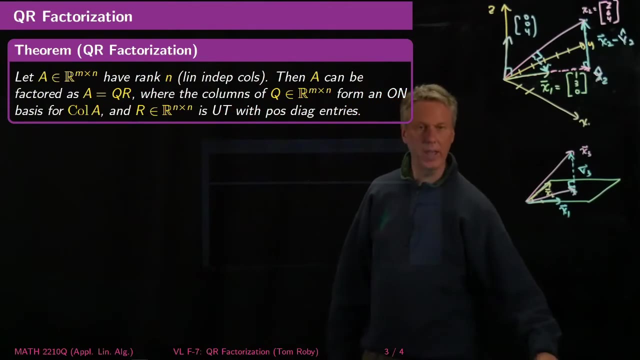 to get Q is just by, exactly by using Gram-Schmidt orthogonalization. I'll just take the columns of A and Gram-Schmidt them so that I get the columns of Q. Now R will have these other properties, It'll be an upper triangular matrix and it'll have positive diagonal entries. 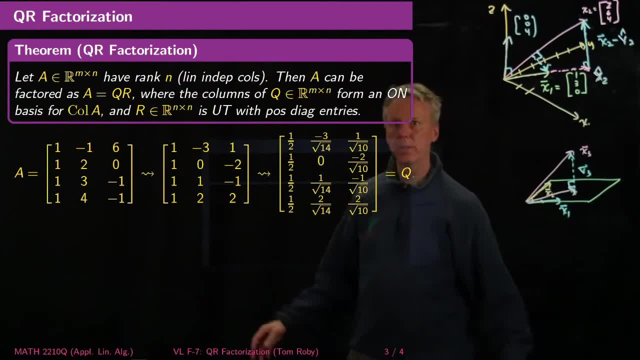 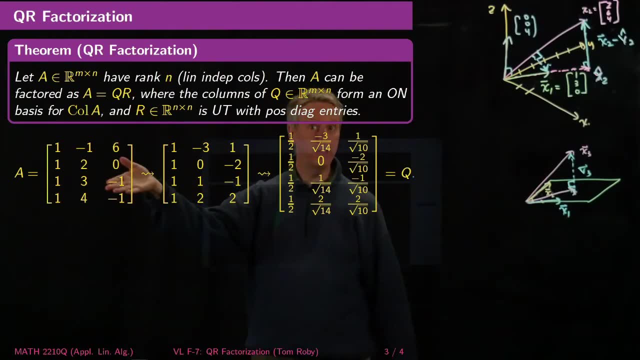 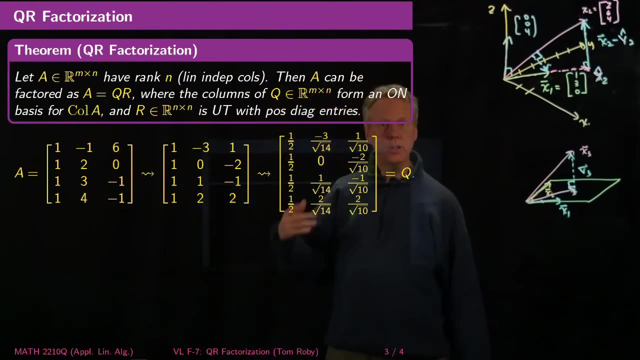 So let's see immediately on an example how this works. So here I've got a 4 by 3 matrix. So M has to be bigger because these three columns have to be linearly independent, which means that we have to be in at least R3.. Here we're in R4. And the usual Gram-Schmidt algorithm. 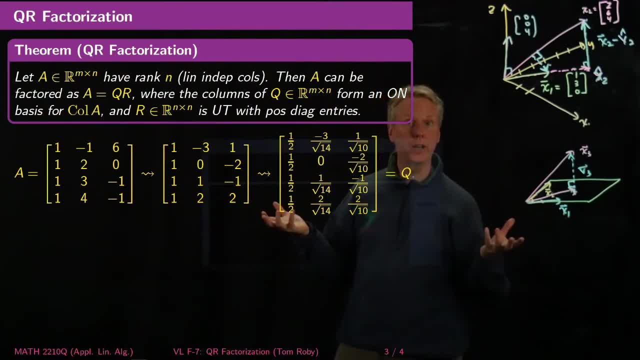 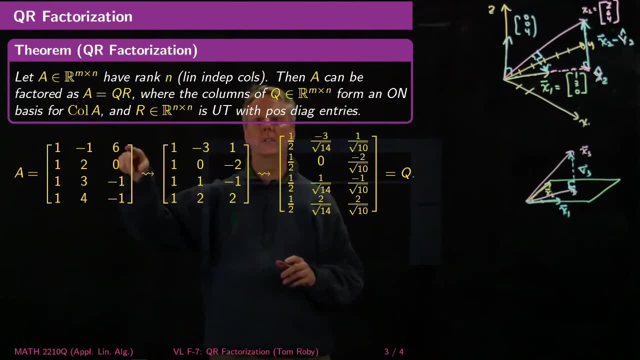 I'm not sure it's worth showing it to you again right now, but you might want to check at home and double-check my arithmetic. make sure this is correct: that if you Gram-Schmidt these guys, these three vectors, then you get these three vectors. How do you see that? 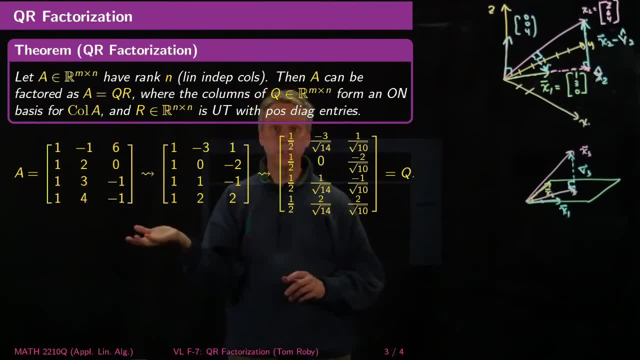 Well, I mean the first column should be the same right, And then the second column I should get by 3. Taking, by projecting this vector onto that vector and subtracting it from this vector, So I should have minus 1,, 2,, 3,, 4. And I should be subtracting from it some multiple of 1,. 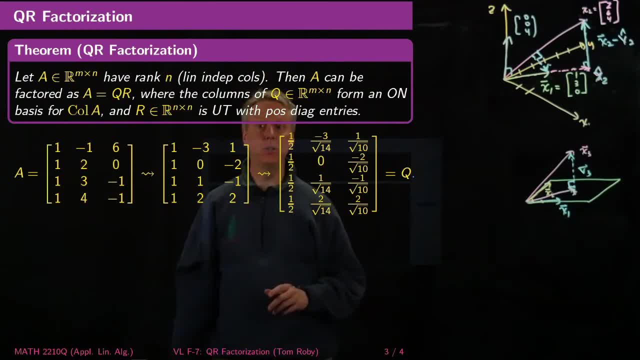 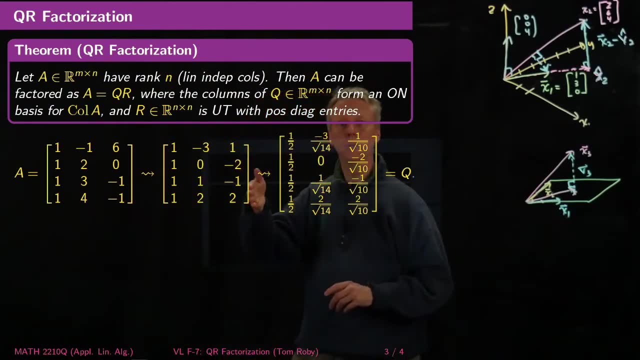 1, 1, 1.. In fact, that multiple of 1, 1, 1 turns out to be 2.. And so that's why I get negative 3, 0,, 1, 2.. And similarly, you project this onto the subspace band by the other two. 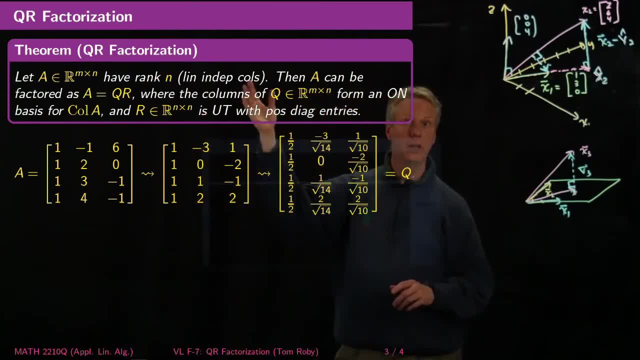 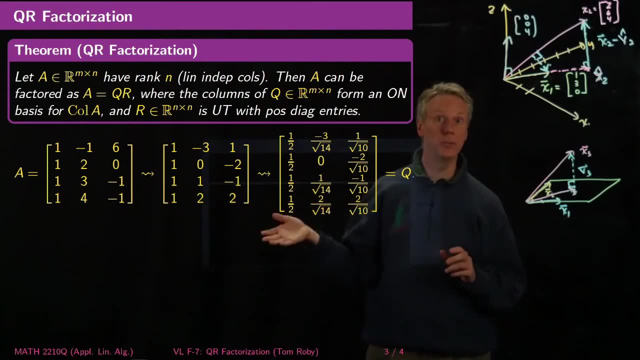 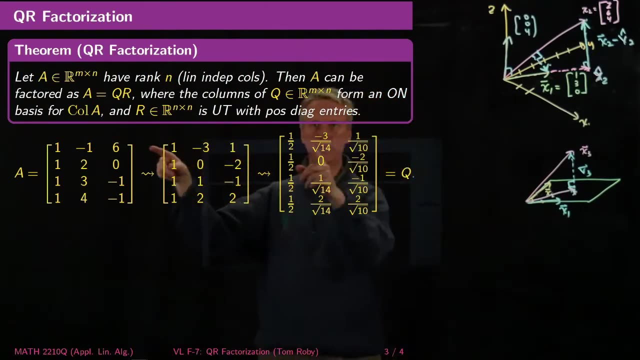 And so you get this nice orthogonal, A set of three orthogonal vectors. Now remember that a matrix is not orthogonal if it has orthogonal columns. It needs to be square and have orthonormal columns. And here we don't even have a square matrix, But we do have. it's now orthogonal And you can just. 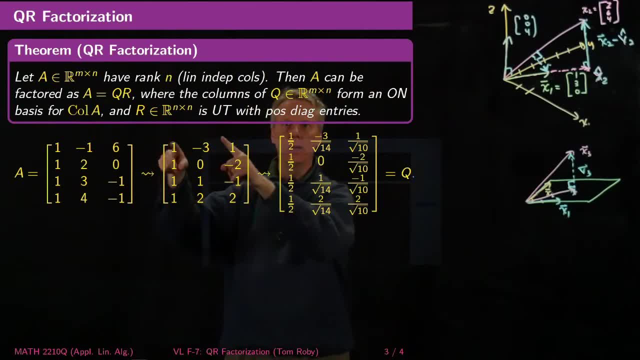 check at least that that's true. right? That's easy to do, because here we'll have minus 3 plus 0, plus 1 plus 2. So that dots to 0. Here we get 1, minus 2. So I've got minus 1.. Another. 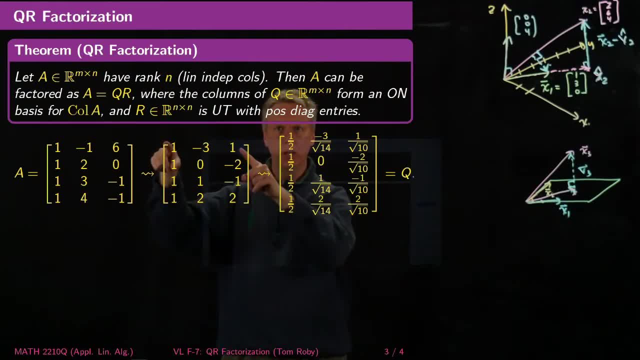 minus 1 is minus 3.. 1, minus 2 is minus 1, then another minus 1 is minus 2, plus 2 is 0,. good, And now here I'll have minus 3, 0,, still minus 3,. 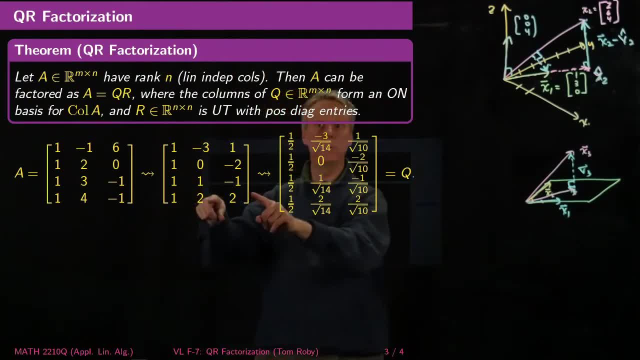 so then minus 3 minus 1 is minus 4, plus 2 times 2 is 4, good, So there's some good chance that I did that right, because at least in the end I got a basis that was orthogonal. 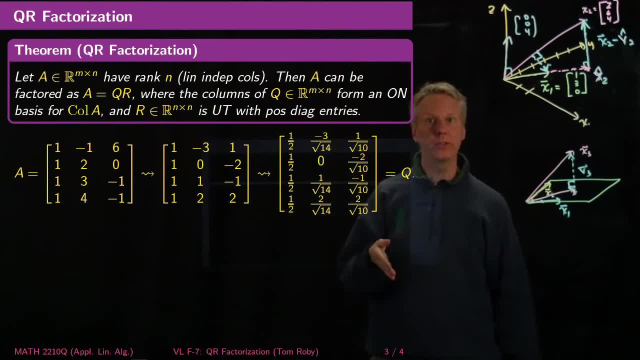 And now I just normalize each of these vectors by dividing by its norm. So the norm of this is the square root of 4, which is 2, so I'm dividing by 2 everywhere. so this vector is all a half. Here I'll be dividing by the square root of 14,. 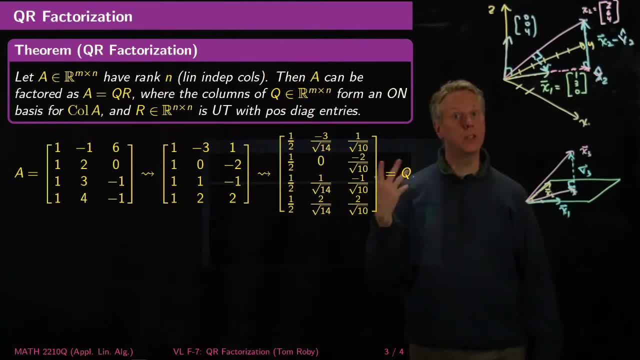 and this last one I'm dividing by the square root of 10.. So that's my matrix Q. It's still the same dimensions, it's a 4 by 3 matrix, but now it's this nice property that the basis that each of the columns, the set of columns, is orthonormal. 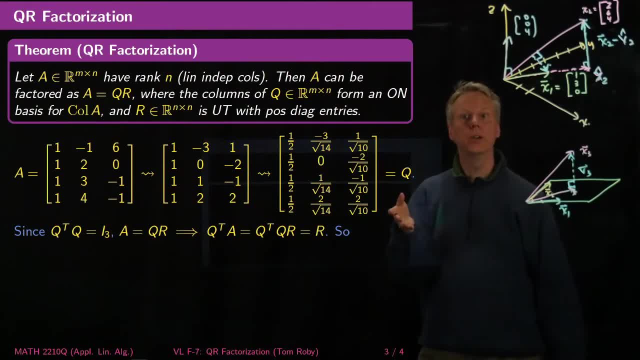 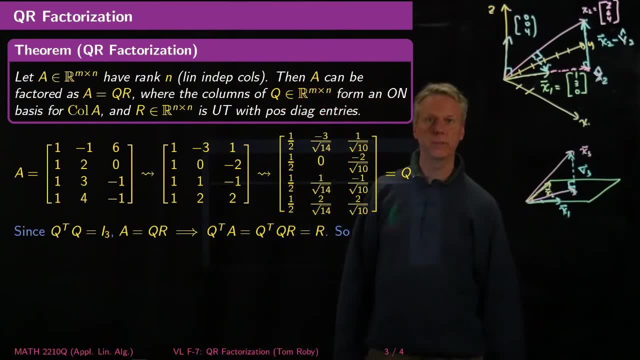 And one of the things we know- when we have a rectangular matrix, those columns are orthonormal- Is that Q transpose times, Q is the 3 by 3 identity matrix. okay, So I mean I found Q, how do I find R? 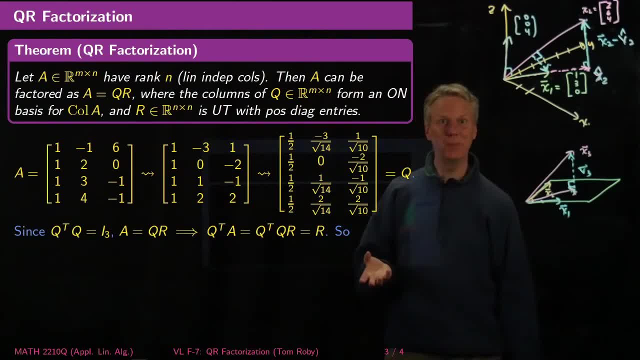 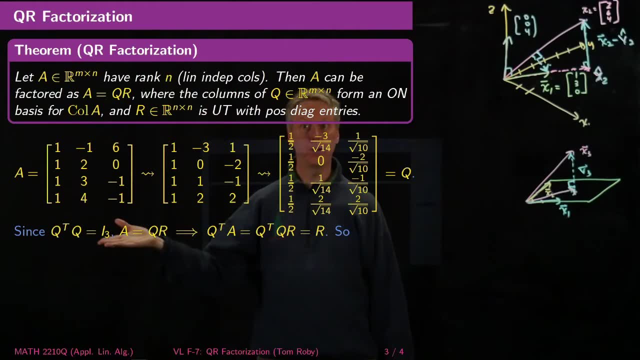 And here's the key thing is that R comes out of this incredibly simple but neat algebraic trick. So if Q transpose Q is equal to the 3 by 3 identity matrix. if I want to find A, equals Q times R, and I found Q. 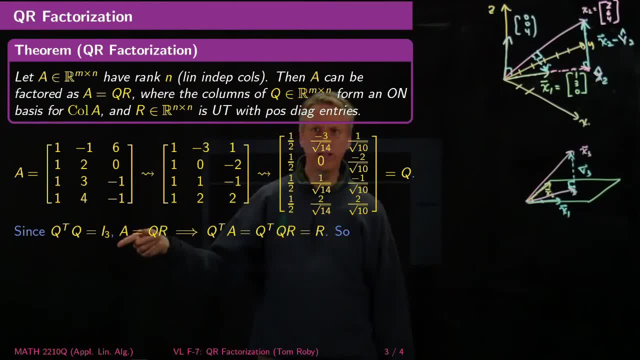 and I know A. how can I get R? I can't divide by another matrix generally, but here basically, Q transpose has given me a one-sided matrix inverse And so I can just multiply both sides of A equals QR of this equation. I just multiply that on each side by Q transpose. 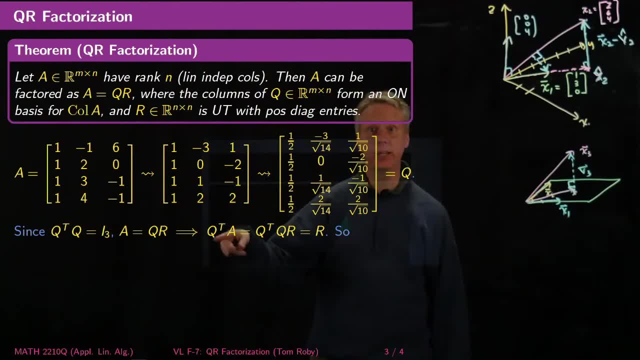 Can't stop me from doing that right. So Q transpose times A is equal to Q transpose times Q times R Associative property still works. So this is Q transpose times, Q times R, and we just say Q transpose times. Q is the identity. 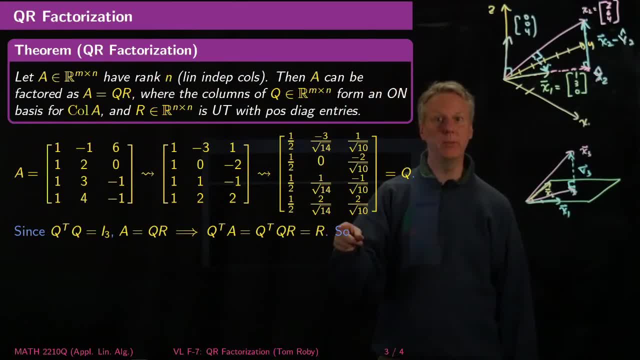 So we just end up getting R. So in other words, the point is that we've computed R now as just Q transpose times A. So we just take the original, we take the Gram-Schmidt matrix, take its transpose, multiply it on the left of A. 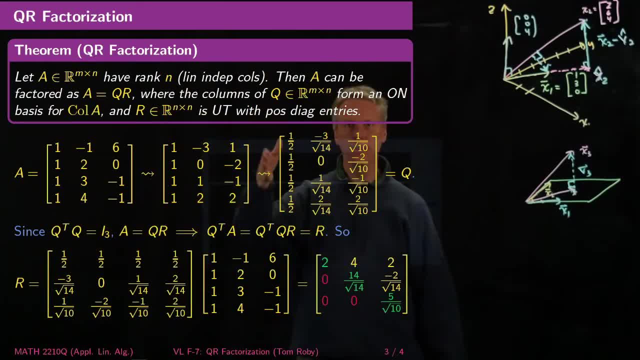 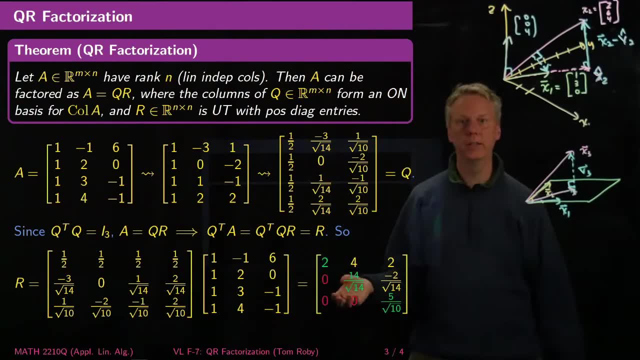 So that's what we get here. That'll give us R. So here, I've taken this matrix, I've taken the transpose, as you can see, And now, if you do this matrix computation, you'll find, lo and behold, that you got zeros below the diagonal. 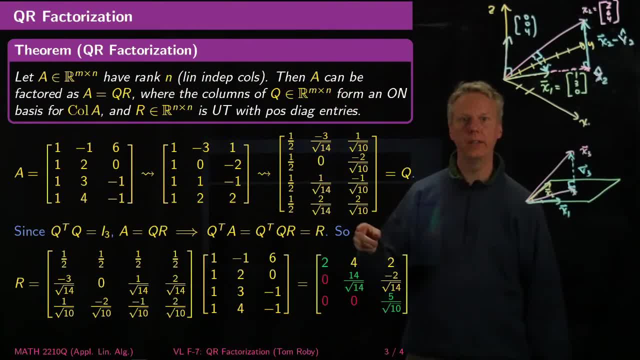 So that's what we get here. We get the diagonal, as advertised, And along the diagonal we get these vectors that I've marked in green, and you'll notice that they're all positive. Okay, So that's how to do the QR factorization in practice. 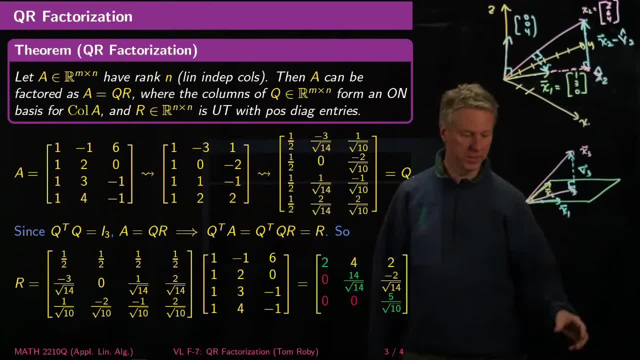 So once you, the hard work is all in the Gram-Schmidt and then the rest of it is just making sure you don't make an arithmetic mistake, because if you're doing it by hand, you probably have square roots in the denominator. 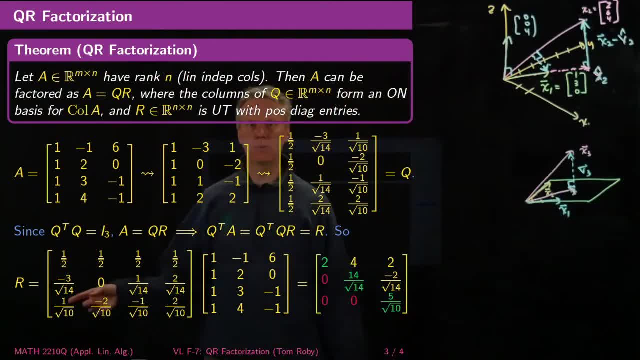 But notice that the square roots don't really bother you in the sense that it's the same square root everywhere, right? So, for example, if I wanted to check that, say, that middle entry is 14 over the square root of 14,. 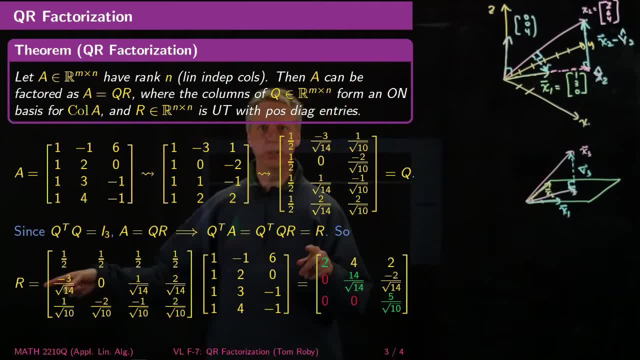 which I could have simplified to the square root of 14,, but there was no real advantage here to doing that. then what do I do? So here I have, you know, 3 over the square root of 14 plus 0,. 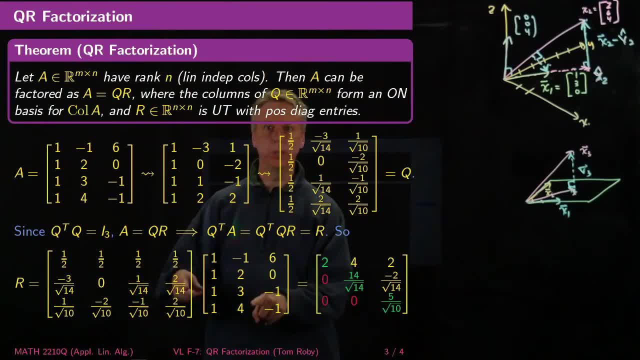 plus 3 over the square root of 14.. So that's 6 over the square root of 14 plus 8 over the square root of 14.. So it's really 14 over the square root of 14.. I'm really just doing integer arithmetic. 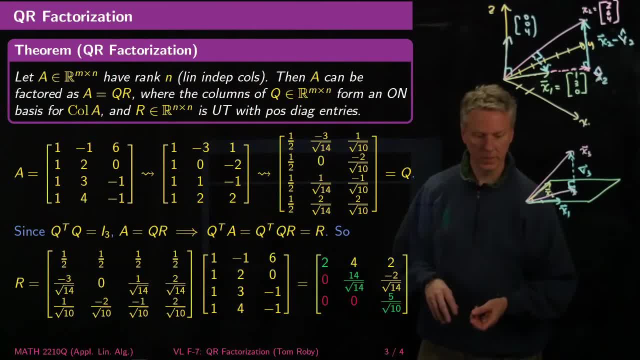 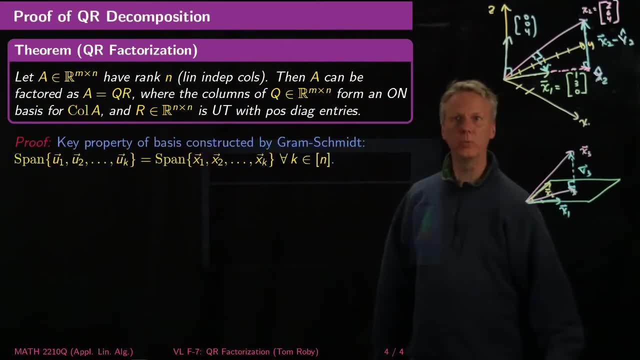 and carrying my denominators along for the ride. okay, So that's the QR factorization, but why does it always work And why, in particular, did we get those? you know, the zeros below the diagonal and the positive actors on the diagonal. 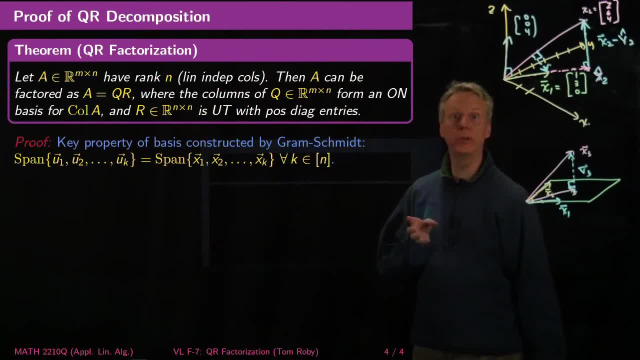 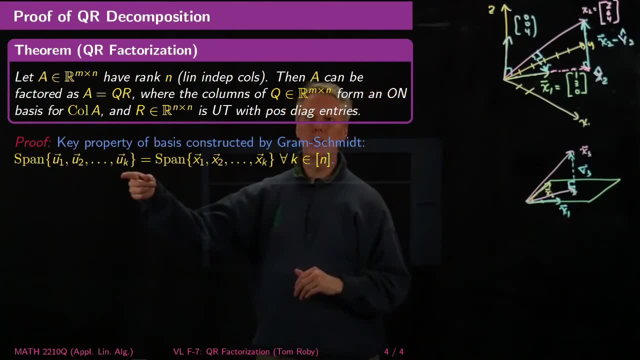 And the key thing, there is this property that we made note of when we were looking at Gram-Schmidt, which is that at each stage of the process, it was always true that the span of the first k vectors. so now I'm saying: 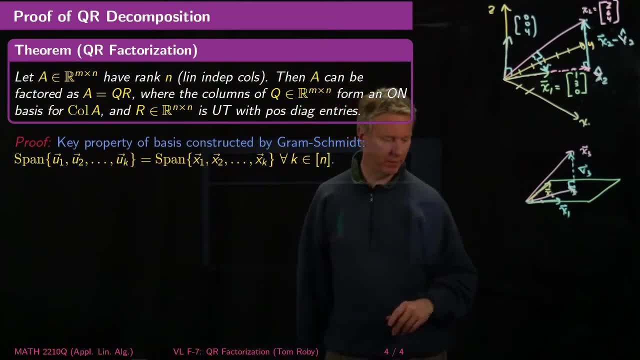 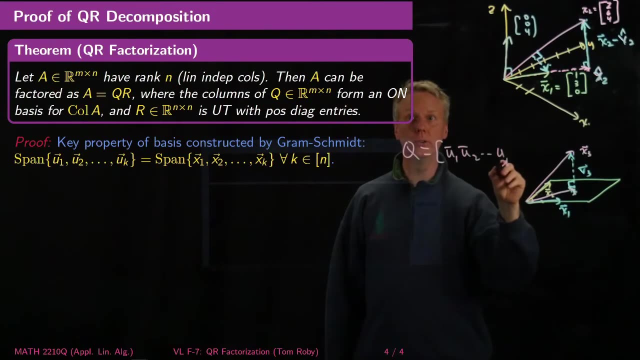 calling u1 through uk are the vectors that I'm creating via Gram-Schmidt, and I want to think about my matrix. Q then is going to be the matrix u1, u2, uk, you know u. I guess I've got n columns. 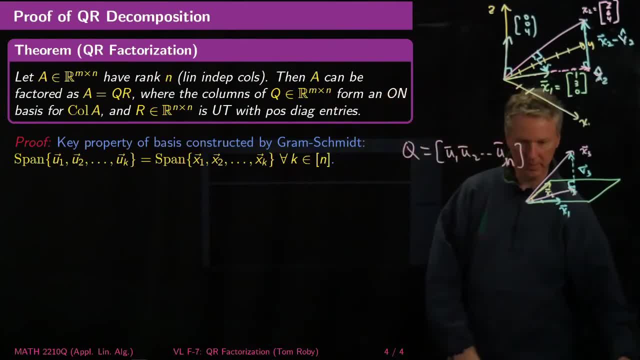 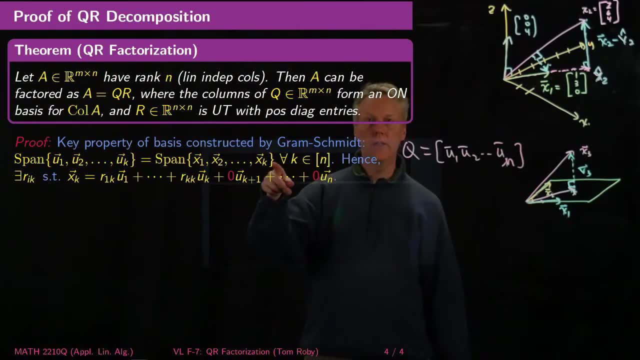 So it's u1 through un. okay. So what does that mean in practice? Well, that means, in particular, that I can write x sub k in terms of u1 through uk. I don't need any, I don't need the rest of them. 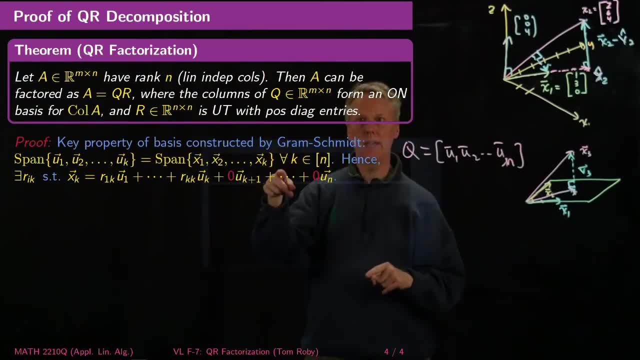 I only need to go to the kth one to write xk. So that means I can write as a linear combination. so I just do that. I write it as r1k u1 plus dot dot dot plus rkk uk, so each. 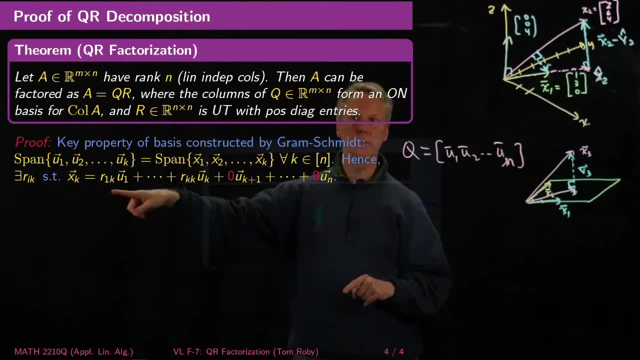 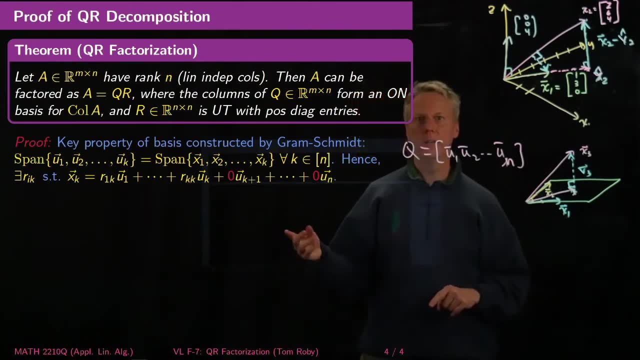 of these scales, The scalars that I'm writing is just r something k r something k times the corresponding u sub i. okay Now, in terms of the whole basis, since I really have n of these things at the end of the day. 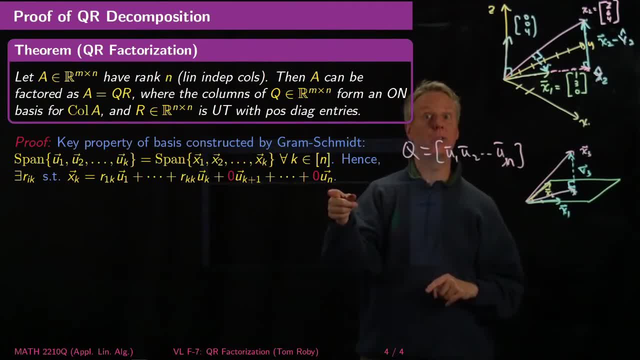 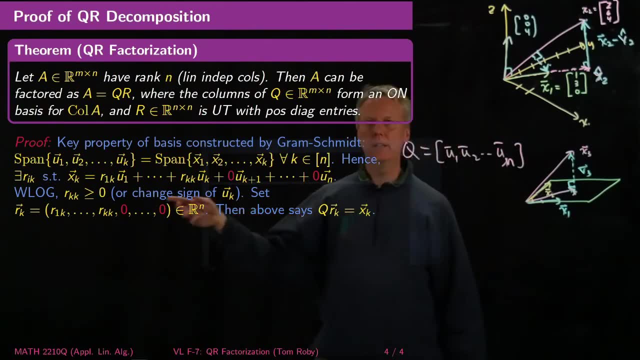 that means I really have plus 0 times uk, plus 1, plus dot dot dot, plus 0 times u sub n. okay, But what that means? oh, and I should say that you know, r sub kk has to be bigger than or equal to 0,. 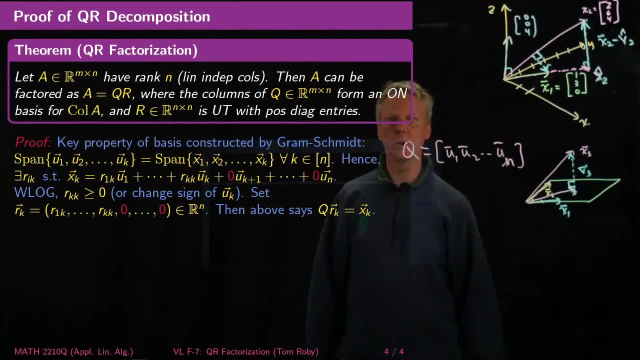 or I could just change the sign of u sub k to make sense. I could just make this work. So and I'll always so, I'll always do that. You know, if I need to change the sign on some u sub i. 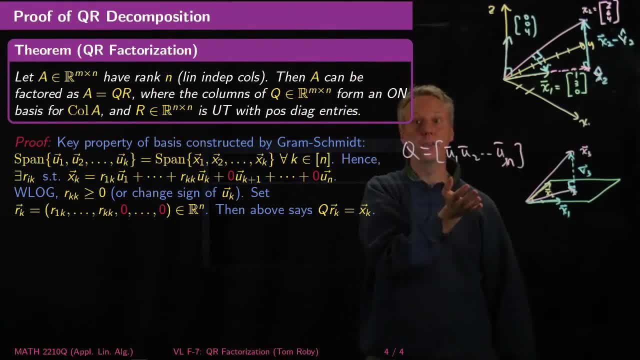 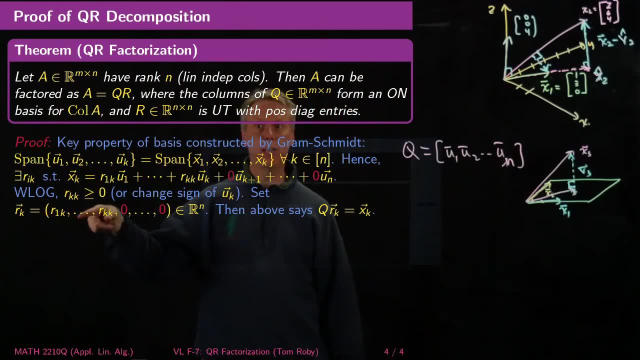 in order to make sure that I have positive things on the diagonal, then that's what I'll do. Alright, so now let's just set r sub k to be this: this is really a column vector: r sub 1k. it's the coefficients on this linear combination. okay. 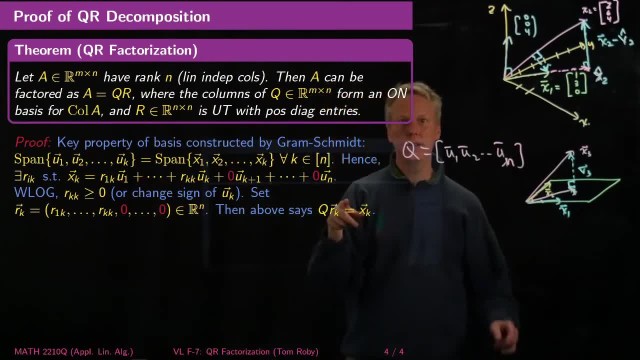 And what this expression is really saying then is that if I take q, which is this set of vectors, and I take the linear combination of that given by this vector, r sub k, that I get x sub k. okay, So that's what this equation says, right? 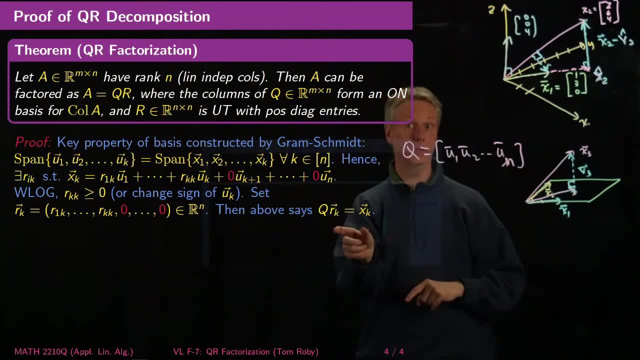 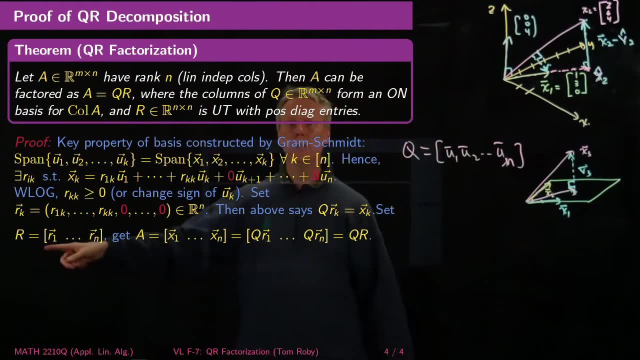 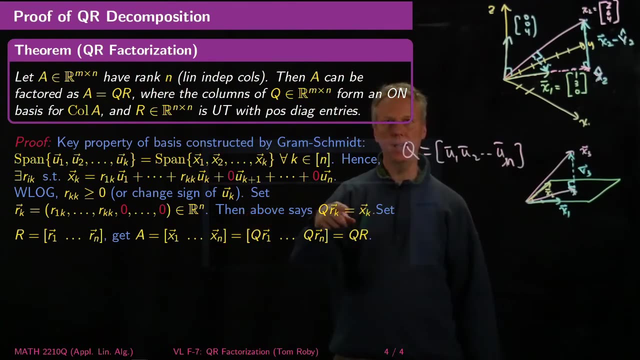 It's just a translation of this equation into shorthand, Okay, but now we're basically done, because now all I have to do is to let r be the matrix of all these r's, So I'll get. I got that. each of these x sub k's. 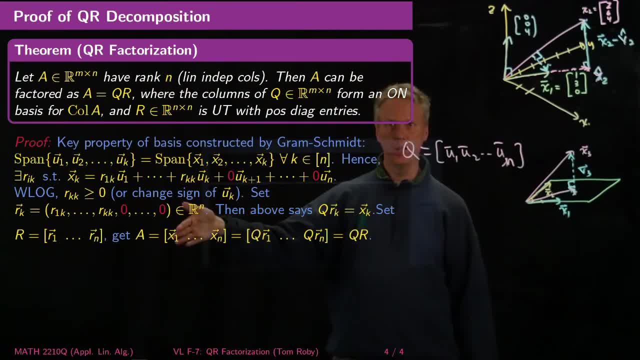 was equal to q times r sub k. so that means that if I put them all in a matrix column by column, that column by column x1 is qr1, dot, dot, dot, xn is qrn. so that's just equal to q times r. okay. 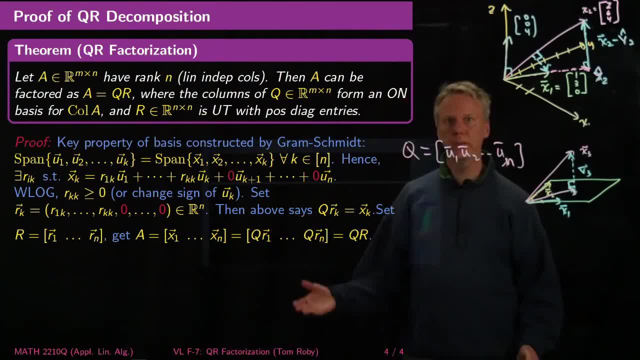 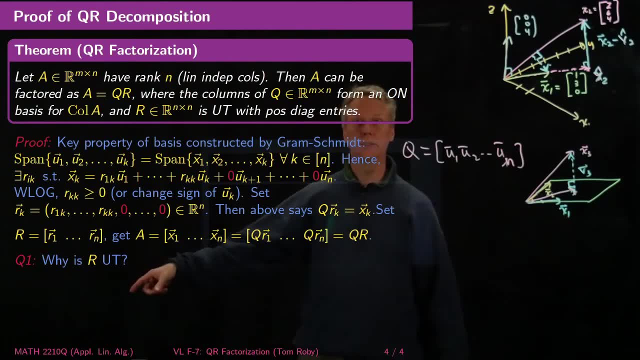 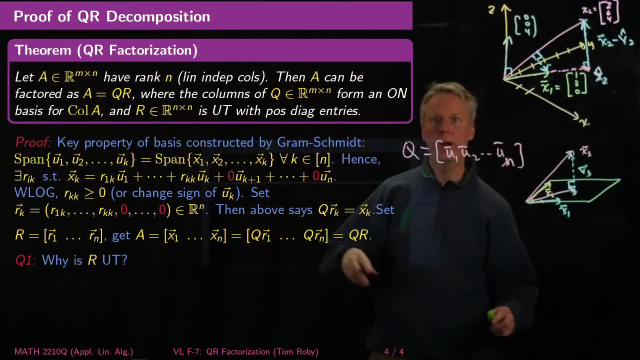 So there it is. it's just a, it's just an easy thing to see, and I guess you might ask a few questions like: first of all, why is r upper triangular? Well, that's this property, right, This property that that says that when I write down r, 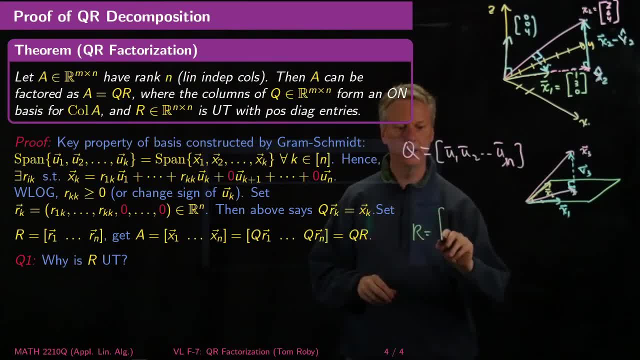 so maybe I'll write a little bit here. when I write down r, so to write down x1, I'll only need r11 times u1, and all the other ones will be zero. So that means if I'm thinking about writing x1 in terms 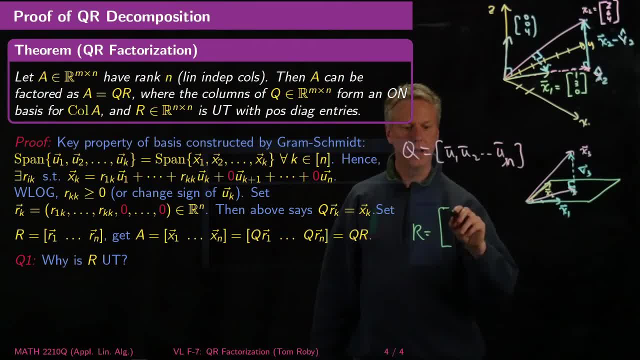 of this basis that I'll only have r11 here and then everything else will be zeros. okay, Now for the next one, I'll need an r12 and an r22, but all the rest will be zeros. and then I just keep going like that. 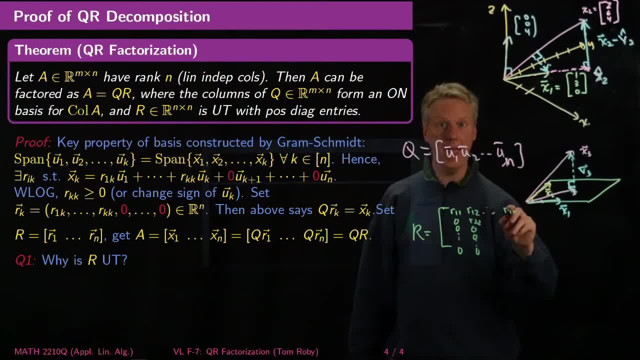 For the last one, r1n. I'll actually need r2n. I might need to go all the way, but all of these guys will be zeros, okay. So that's why it's upper triangular. it's just the construction. 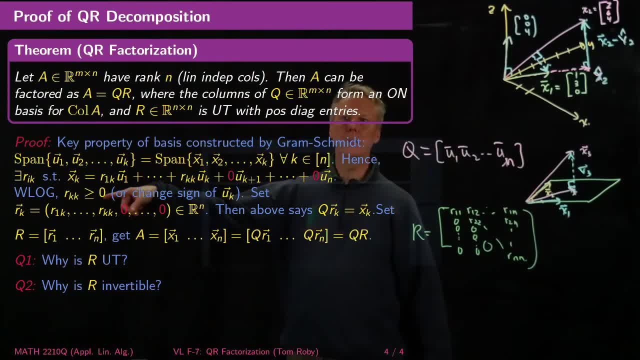 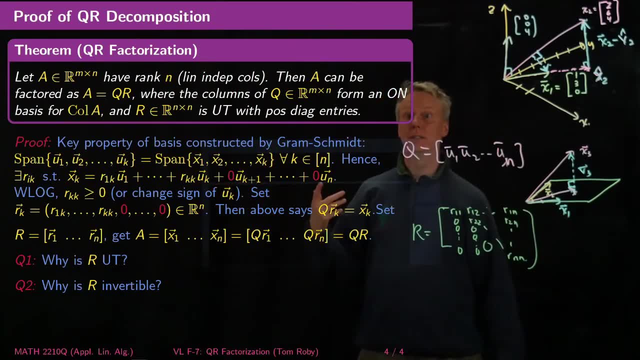 Why is it invertible? So I said I could assume that r sub k k was bigger than or equal to zero, and maybe I could make an argument just in the middle of this to show that r sub k k had to be greater than zero. because well, 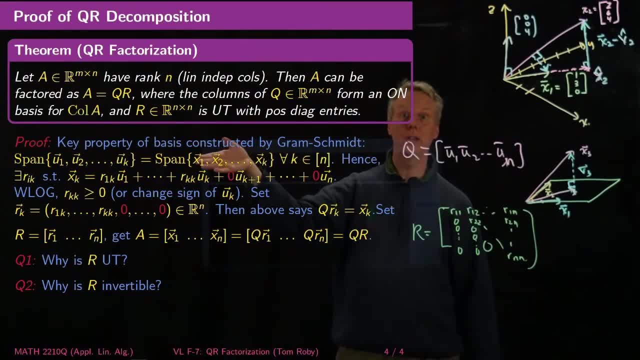 I know that these guys are linearly independent, right? So that you know I'm going up a dimension every time I add an x sub k, which means I need to. you know I'm going up a dimension every time I add an x sub k, which means I need to. 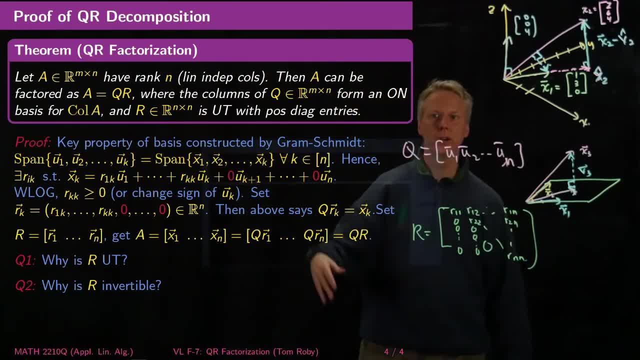 go up a dimension every time. I add a u sub k, which means that coefficient has to be non-zero. But there's another way to argue it, which is just from the way qr works. And this is kind of nice because it's helpful to think about things this way. 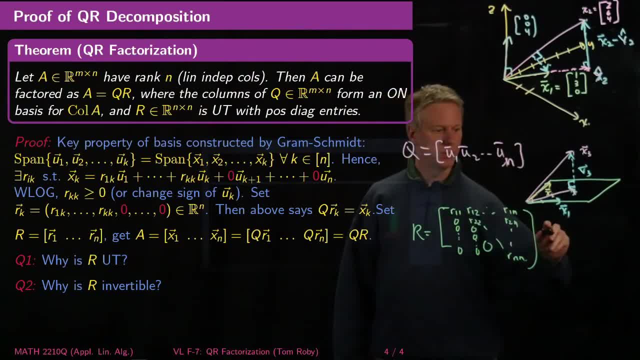 So why is it invertible? Well, if I think about so, I'm trying to think about a as being equal to q times r, right? So what does that mean? And a is a. we decided what its dimensions are, right. 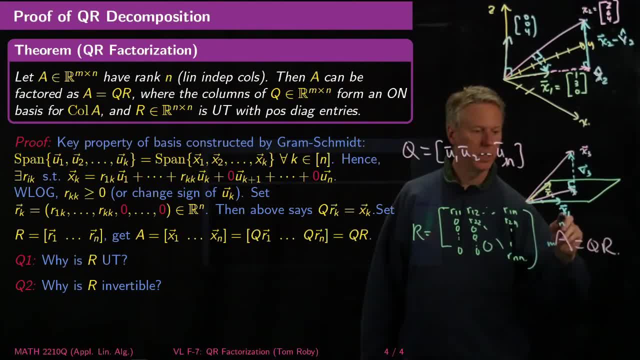 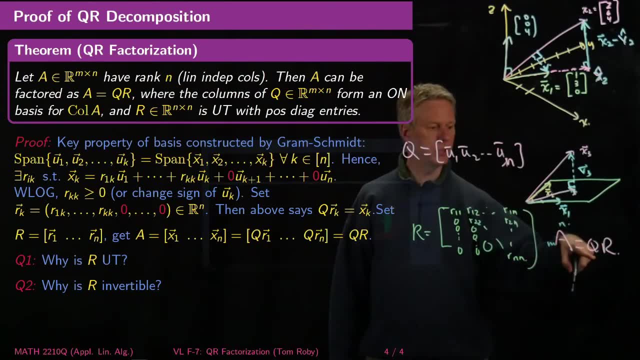 A is an m by n matrix, which means that it represents a linear transformation that's going from rn to rm. Now q is also going from rn to rm, and then r is just going from rn to rn. So what does that mean in terms of my blobs? 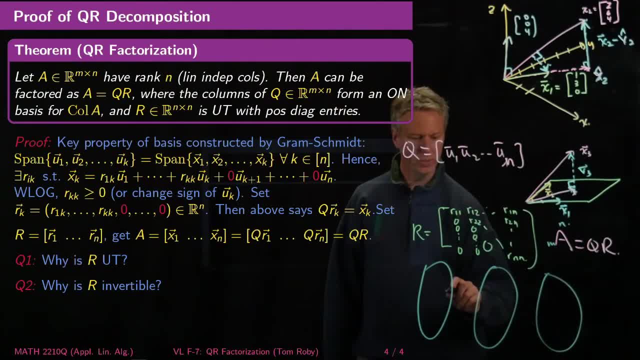 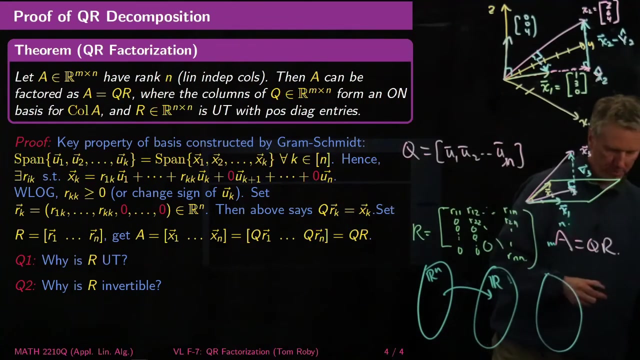 So that means that q is going from r to the n to r to the m, and then a right. Not quite right, because when I do a equals qr, I do r first. Okay, so what that means is that I need to do. 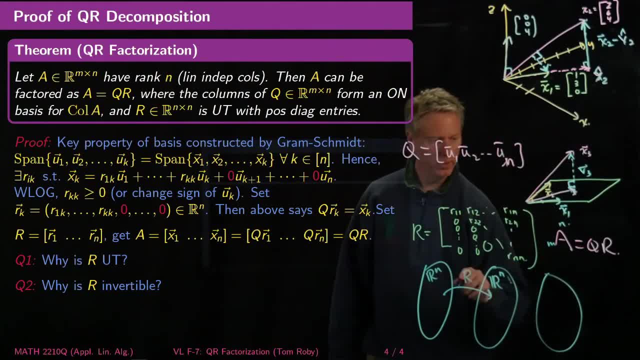 r is going to go, r is going to go. r is going to go. this matrix, r is going to go from r to the n, to r to the m, and then it's followed by q, which goes from r to the n to r to the m. 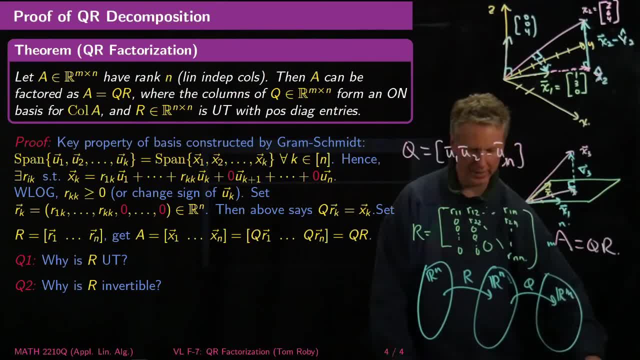 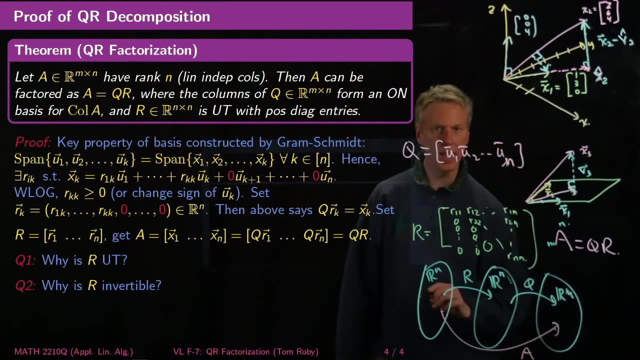 So a, on the other hand, is: this is the combination of these things, right? So this is the same as the transformation a which goes from r to the n to r to the m. Okay, so now how do I show? 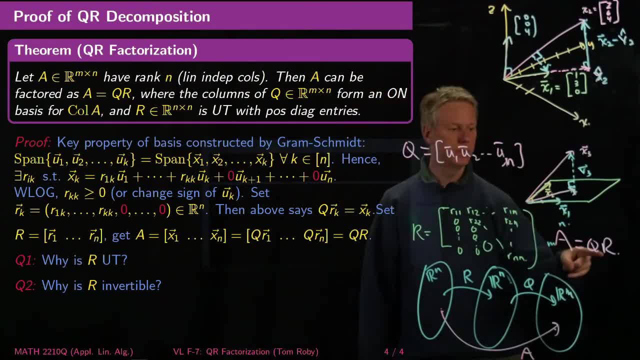 how do I show that? how do I show that r is invertible? Well, if r wasn't invertible, then what would happen? If r wasn't invertible, then, since this is a square matrix, by the invertible matrix theorem. 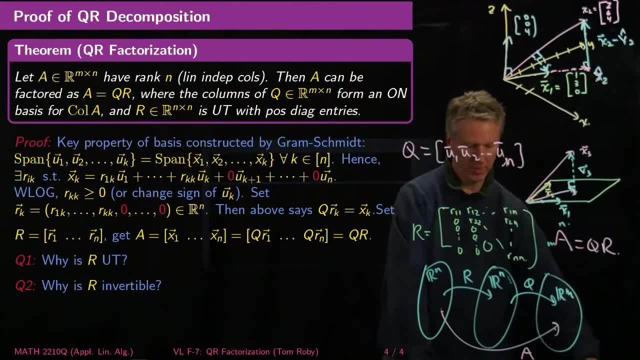 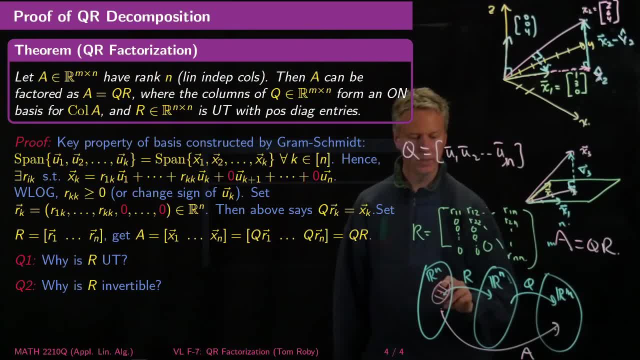 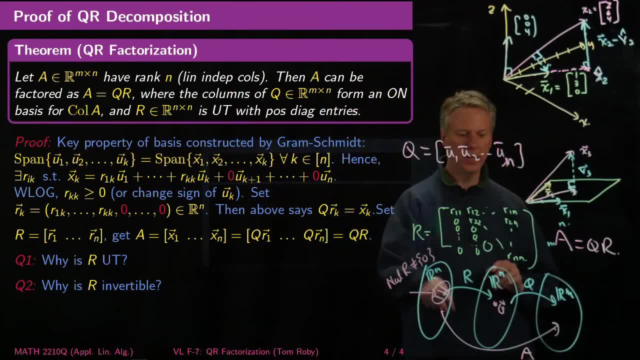 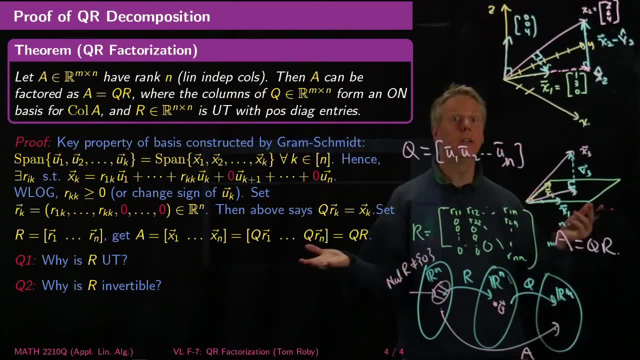 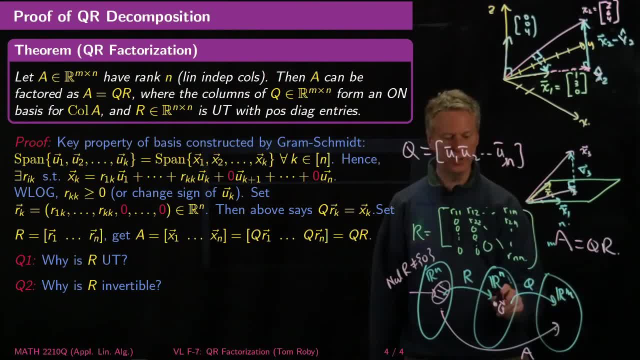 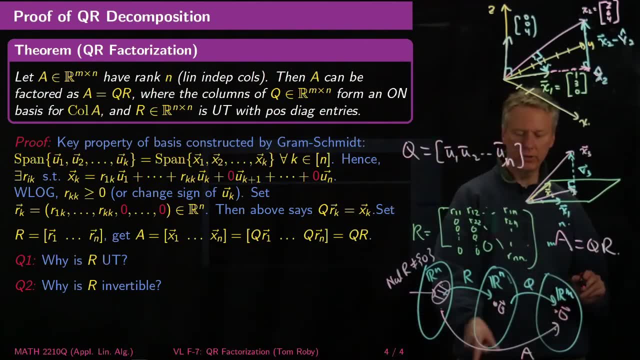 if a is equal to q times R, well then anything that went to 0 here will definitely go to 0 there. So if I have a non-trivial null space for R, then I must have non-trivial null space for A. 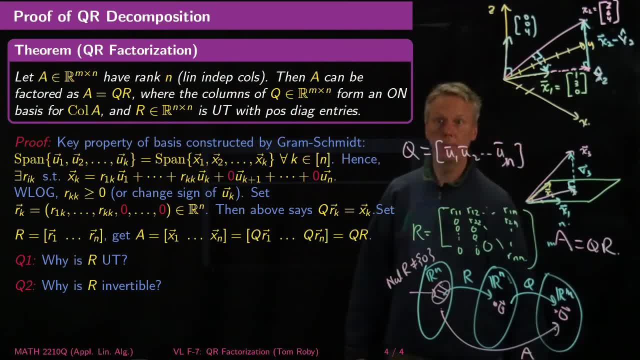 but I don't have a non-trivial. That's one way of seeing that r is invertible. And once you know r is invertible then since it's triangular, so the next question is: why are all the diagonal entries positive and not just? 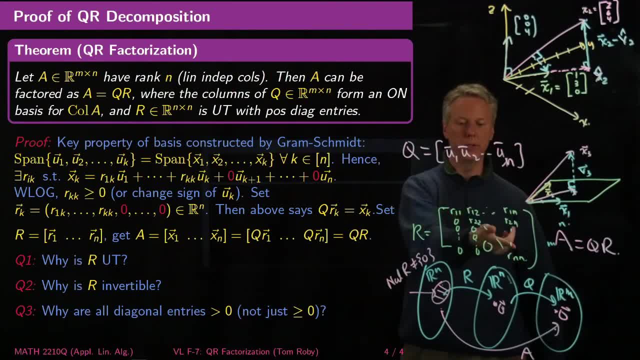 non-negative. Well, if one of the entries was actually 0, then this determinant would just be 0,, right? We know that an invertible matrix has non-zero determinants, so this can't be So. none of those entries can be 0. 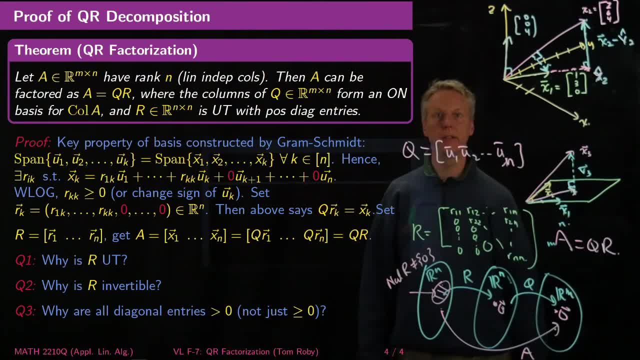 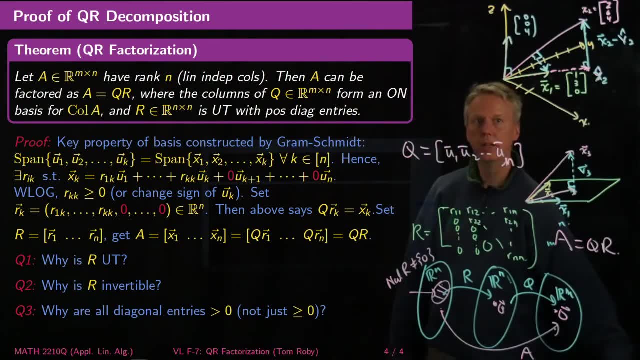 So those are the answers to those questions, and I think that's it for QR factorization. It's just a nice way of thinking about Gram-Schmidt, but it does have applications where you use the QR decomposition of a matrix to do certain kinds of computations involving 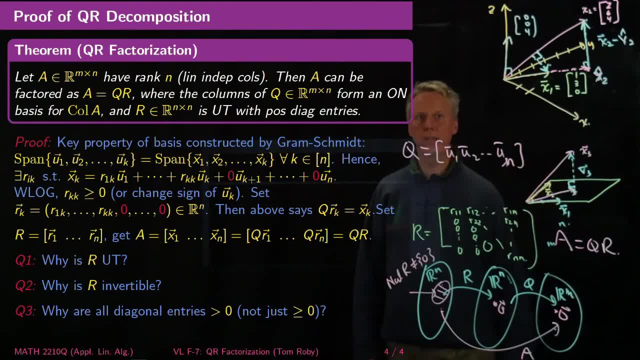 for example, least squares, which we're going to get to soon. So that's it, Thank you. Thank you for your kind attention.